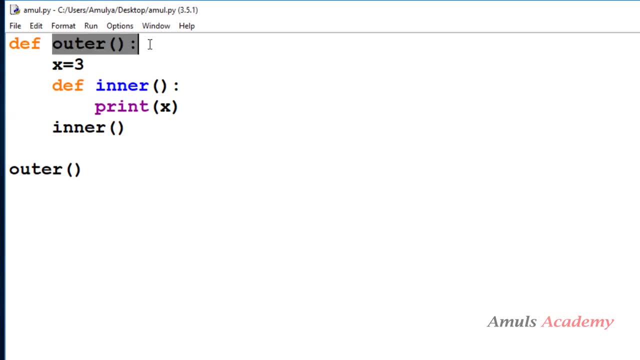 here we can see, Here this outer function is the enclosing function, This inner function is the nested function, because this function is inside another function. right, And here this nested function can use the enclosed variables or the names which are defined in the enclosing scope. ok, this is the enclosing scope. ok, here x is equal to. 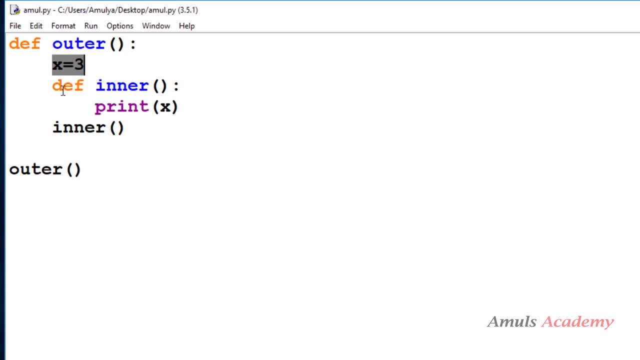 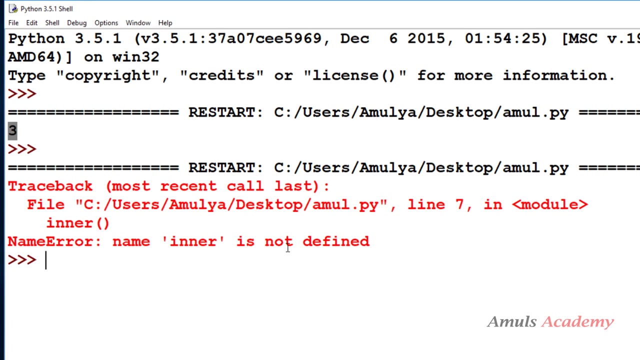 3: this is the enclosed variable. we can use that inside this nested function. alright, this is about the nested function And i can't call this function outside this function body. for example, now here, if i call this inner function, ok, here we can see the error name. error name: inner is not defined. 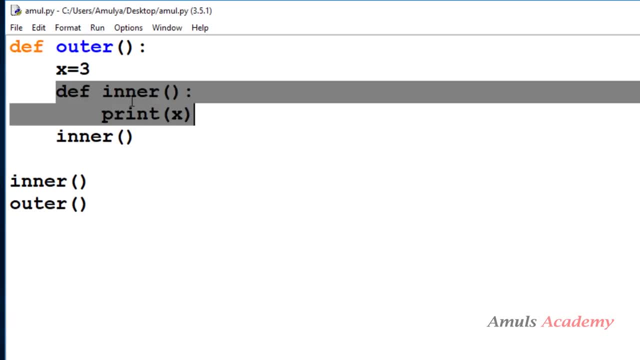 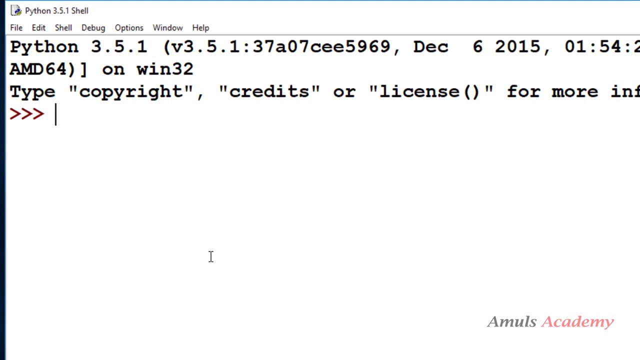 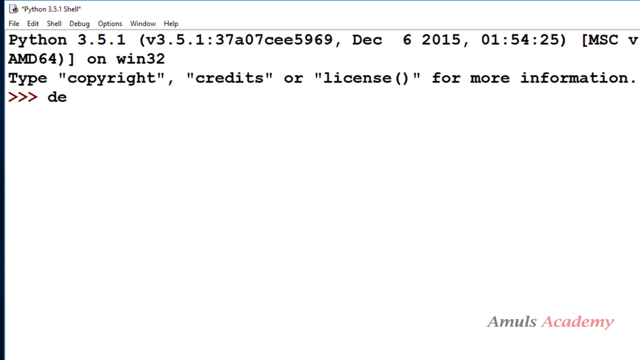 because this is the local function to this function. ok, we can't call this function outside this outer function body. ok, so this is about the nested function. ok. So next concept is: functions are object. so in python functions are object. we can assign a function to variable. that's nothing. but first i will define a function. i will just 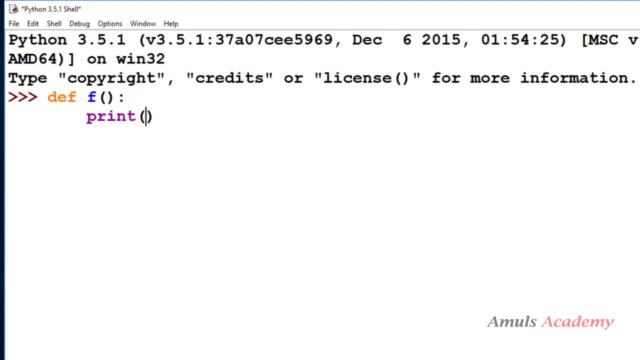 give name as f, ok, and it will just print hi. ok. so now, to call this function, i need to write the function name and parenthesis, right, so it will print the message hi. So now, if i just mention the function name, ok, i won't call this function. to call this: 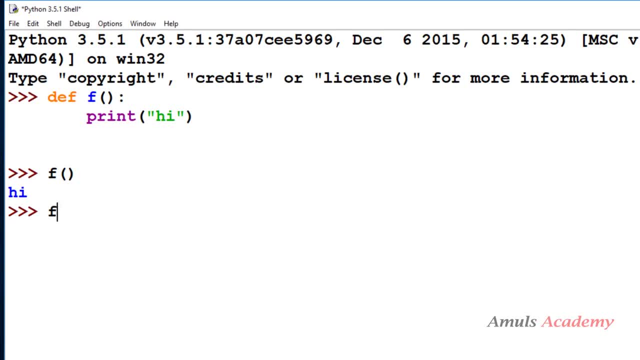 function. i need to use parenthesis, but i am not calling this function. i am just mentioning a function name and if i enter we can see function f at this location. ok, here we can see the function object reference and in python i can assign this to an variable. so if i take 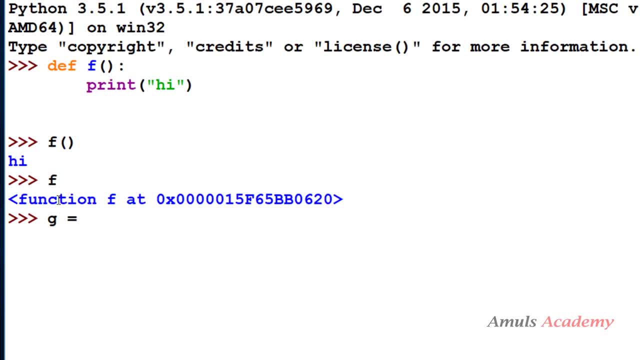 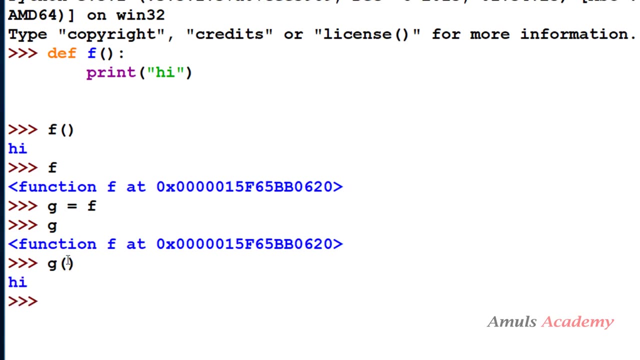 a variable called g. if i take f, ok, g is also same. ok, g is the another name given to that reference. ok, so if i call g now, it will print hi. ok, so if i call a function without parenthesis, it will give that function reference. ok, so now coming to this closure concept. 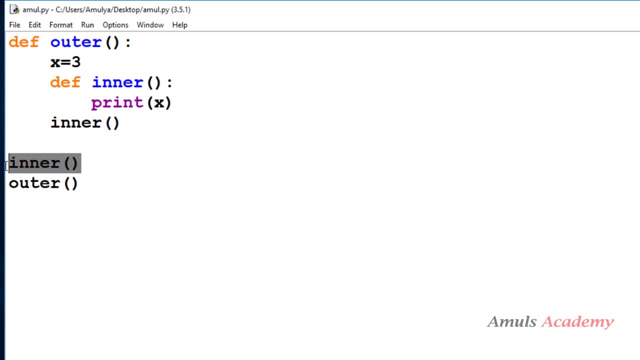 Here. as i said, i can't call this inner function. ok, so i will delete this. so now, here we can see. i am calling this inner function inside this outer function. ok, so now, instead of calling this function, what i will do is i will return this as well as i will call this function. 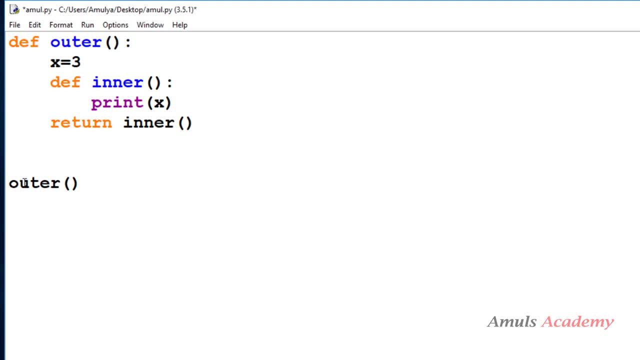 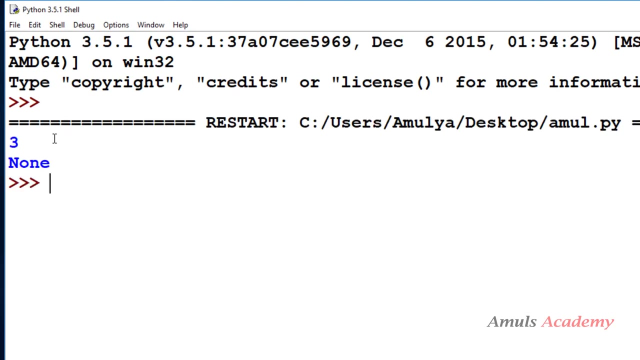 ok, so here i am returning something. that's why here i will take a variable or a name. ok, i will see what it is returning. ok, so i will print that also now, if i save this and run this. so here we can see 3 and none, it is returning nothing. ok, so this is not the value returning. 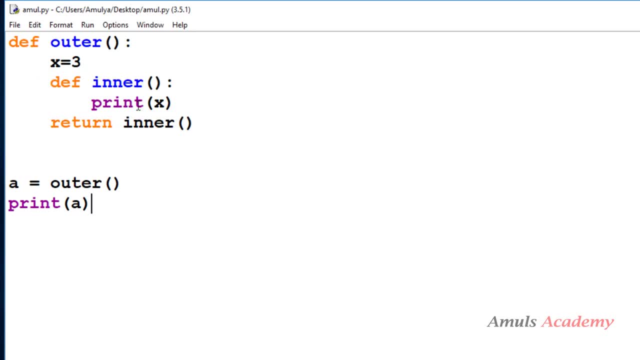 function. that's why it's not returning anything. so if you want to see the value, then i can say: as y is equal to 3.. it will return 6, because here we can see this inner function is returning the result, that is the. it will add 3 plus 3 is 6. it will return that result and it will return that to here. 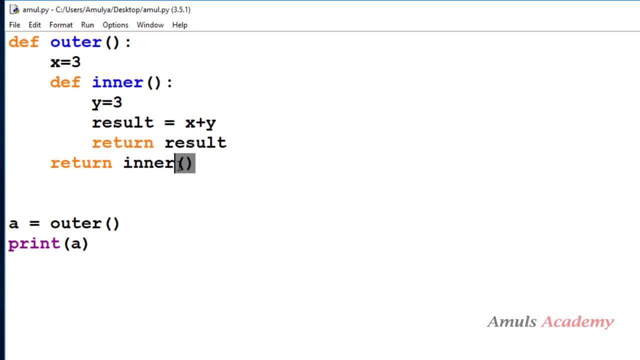 so a value will be 3. ok, so, as i said, if i write a function with the parenthesis, that is function name with the parenthesis, then we are executing that function definition. but if i remove this, so here we are returning the this function reference, inner function reference to here. ok, so now. 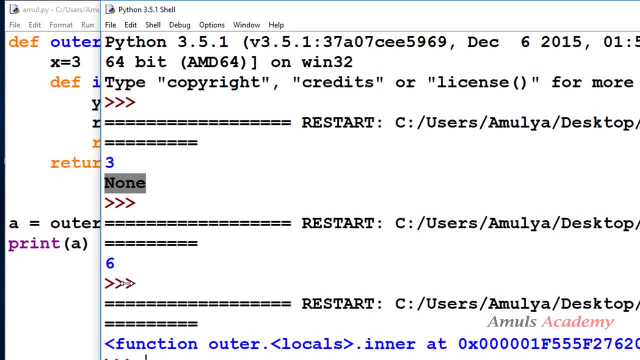 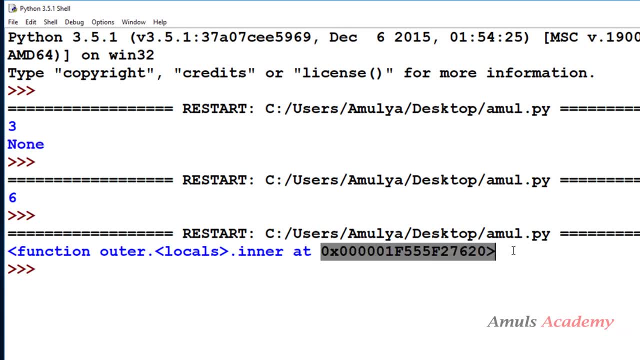 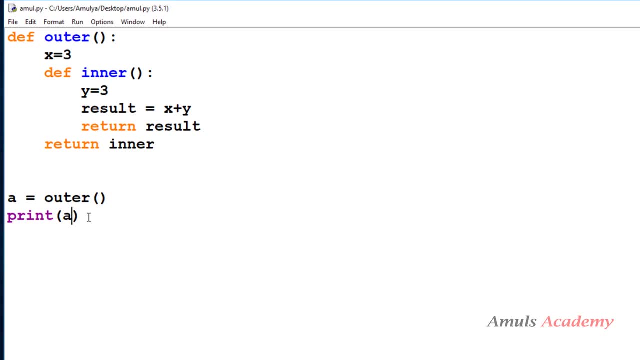 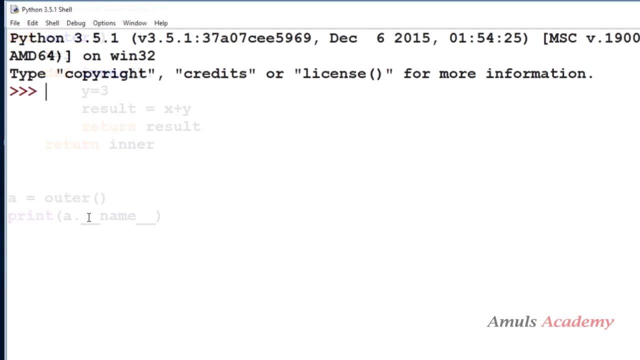 if i save this and run this, it will return this. here we can see function: outer locals, inner, this position: ok, so that is nothing. but if i print the name of a, that is nothing but which function it is pointing to. here we can say inner, so that is nothing, but a is nothing. 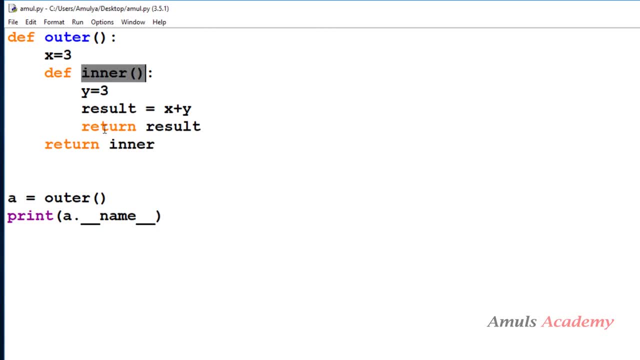 but the inner function. ok, so here we return the inner function reference right, and we are putting the name as a. so that is nothing but a is same as inner function. a is nothing but the inner function. here we can see when i check the name we can see the inner in the. 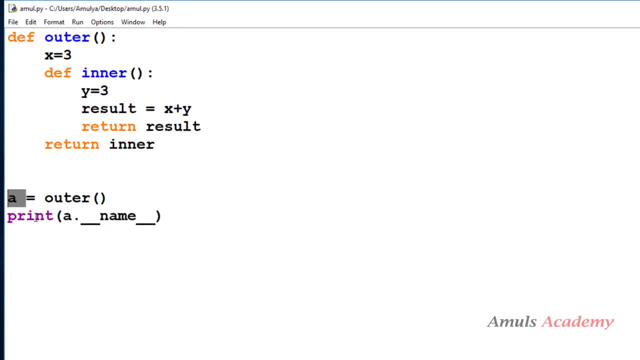 output. right. so here name a and inner are pointing towards the same function. ok, so i will remove this. i don't want to print this now here. i know this a is nothing but inner function, so i can't call inner function here, right? if i call that inner function, i will get name. 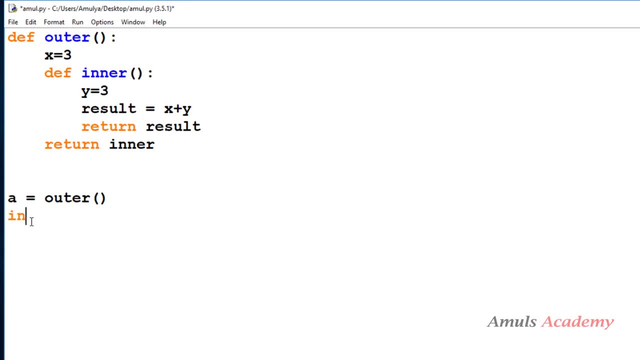 error. we tried that. so if i want to see, we will get name error. so here we know that a and inner are the same, so i will try a here. ok, i will call function a here and if i save this and run this here, we can see. 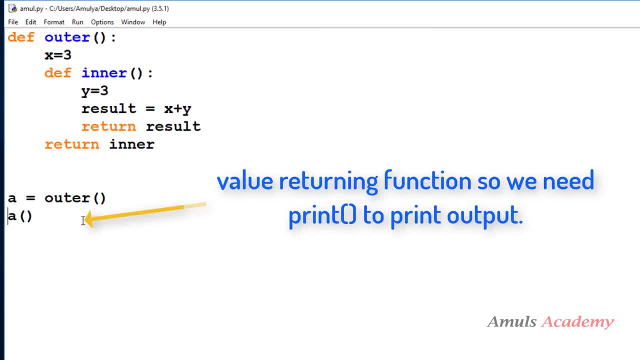 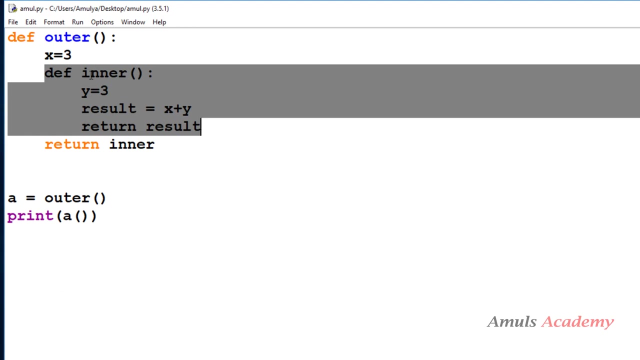 ok. ok, it will return a result. so if i print this, i want to print it right- it will return 6. ok, so that means we executed this inner function body outside its scope. ok, this is the local function. we executed it outside that function. ok, but we know that we can't call an function. 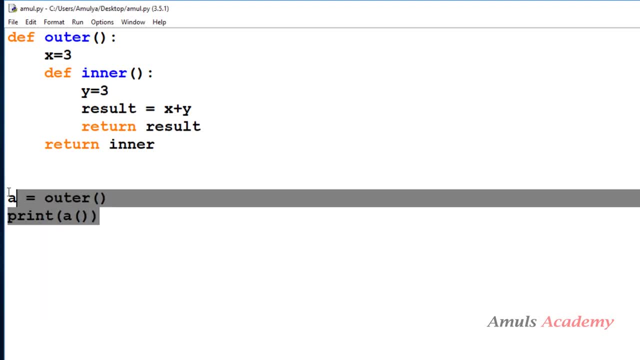 outside its scope, then how we are getting this output. this technique is called as closure. ok, here function a and inner are the same function and we are executing this function outside its scope. ok, this technique is called as closure. the technique by which some data gets attached to the code is called as closures in python. 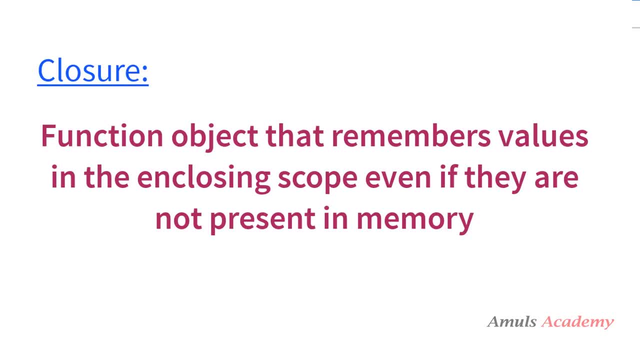 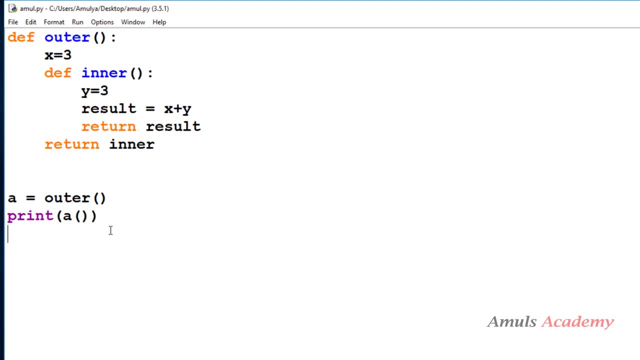 Another definition is: closure: is a function object that remembers values in the enclosing scope, even if they are not present in memory. ok, so this is about the closure. ok, so next i will take another example. ok, so here we can see the outer function, inside that we can see a message, and inner function. 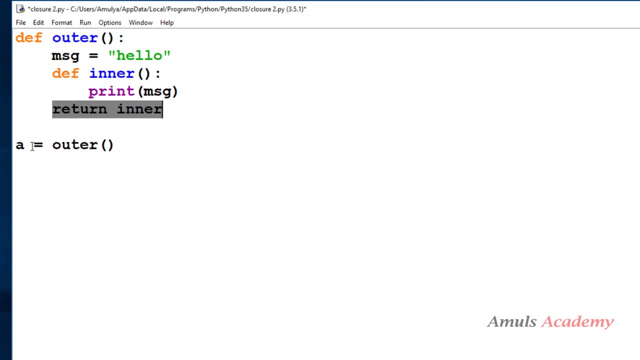 And here we are returning the reference of inner function. ok, and here we can see we took a name, a. ok, that reference will be stored in this and next i will call this function because this inner function is the non value returning function. ok, it will print message. 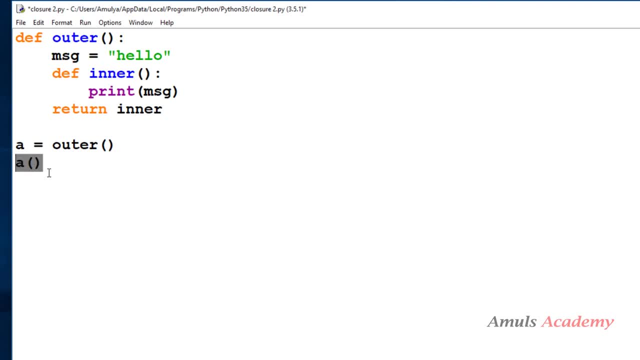 so no need of printing this, so i will just call the function. So now, if i execute this, it will print hello. So here, what happened is We called the outer function, ok, so this outer function will returns the reference to this inner function, right? 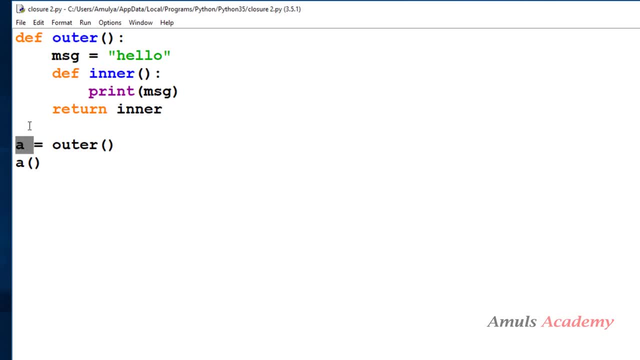 Next, we called this a because a is pointing towards the function inner. we called that and we got the result, even though we finished the execution of this outer function. then also, the message hello is remembered and it is printed: ok, so this technique is called as closure: ok. 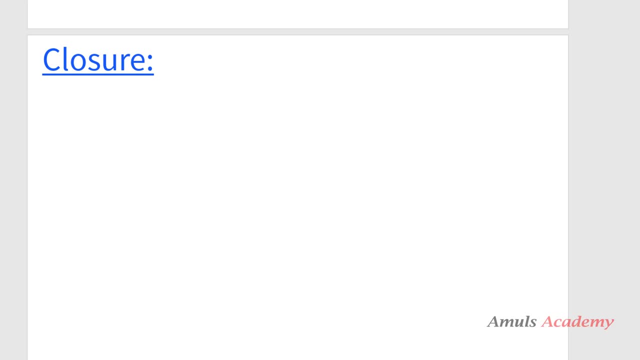 So next question is: When do we have a closure? What are the criteria needed to create a closure in Python? So the first one is we must have a nested function. ok, so that is function inside another function, and the nested function must refers to a value defined in the enclosing function. 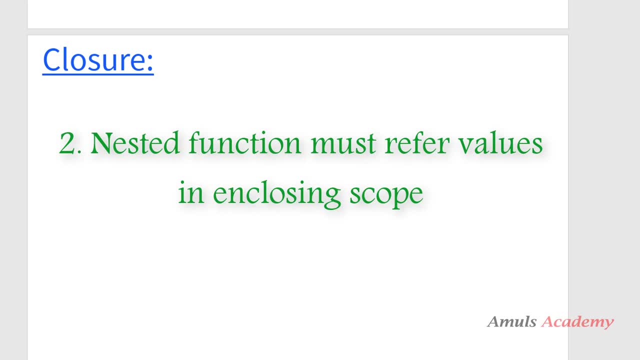 so in the example we saw. so the message was the enclosed variable that was used in the local scope. And the last one is the enclosing function must return the nested function. we saw right. it will return the reference to the nested function. ok, these are the criteria to create. 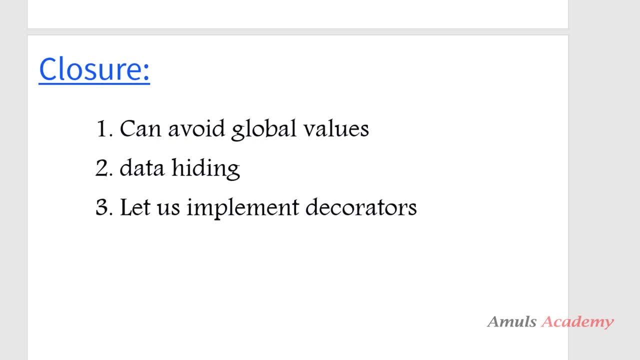 the closures in Python. So next, if you ask what are the advantages of closures in Python? so the first one is we can avoid the global values. here we can see, we call the local function outside its scope, We can point at the enclosed variable outside its scope. right, so we can avoid the global. 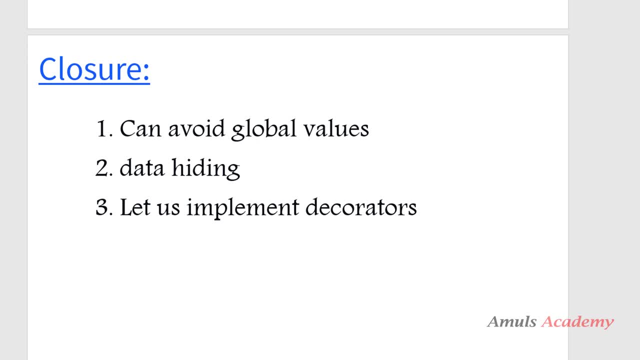 names using this closure. and the second one is it provides some kind of data hiding. third one is it allows us to implement the decorators that we'll discuss in the next tutorial. ok, so that's it for now, guys. thank you for watching. don't forget to subscribe to my channel, i. will meet you in next class. till then, take care.